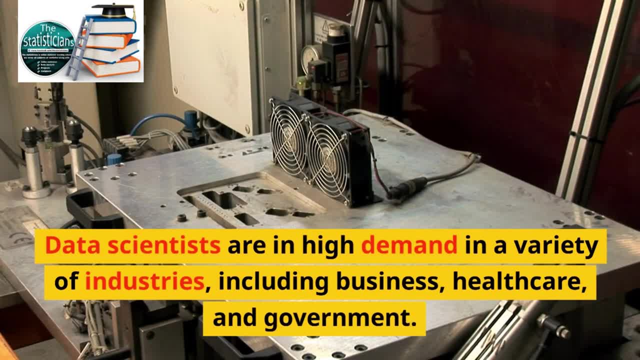 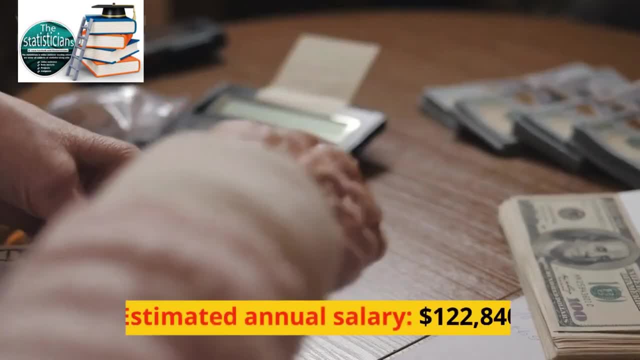 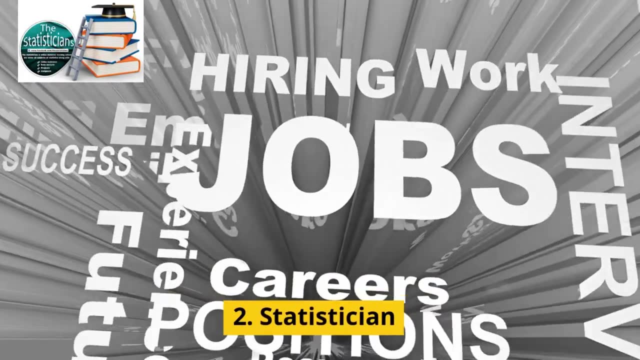 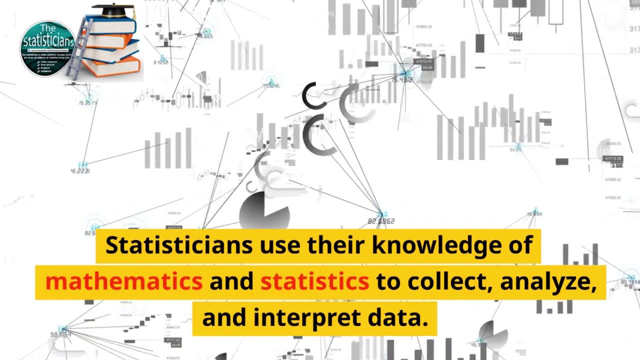 problems. Data scientists are in high demand in a variety of industries, including business, healthcare and government. Estimated Annual Salary – $122,840. 2. Statistician: Statisticians use their knowledge of mathematics and statistics to collect, analyze and interpret data. They use this information. 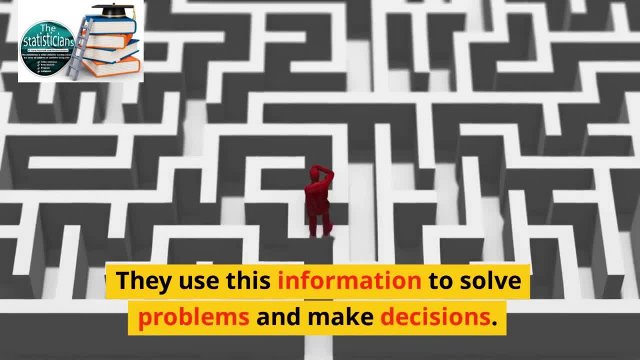 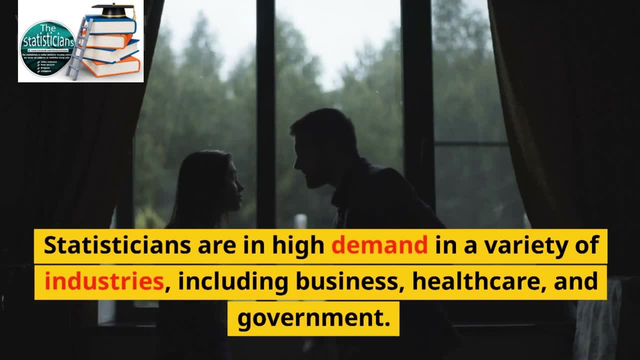 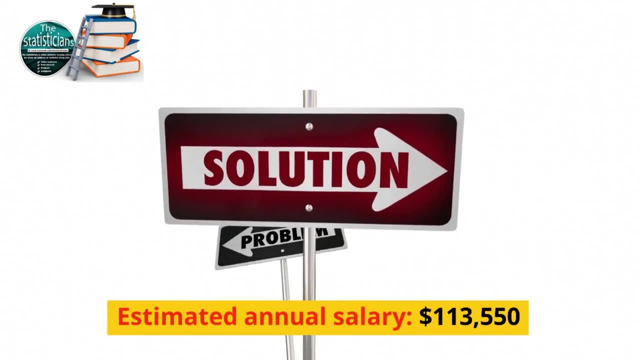 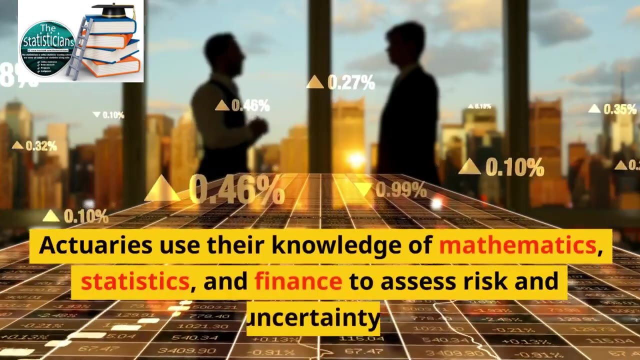 to solve problems and make decisions. Statisticians are in high demand in a variety of industries, including business, healthcare and government. Estimated Annual Salary – $113,550. 3. Actuary: Actuaries use their knowledge of mathematics, statistics and finance to assess risk and 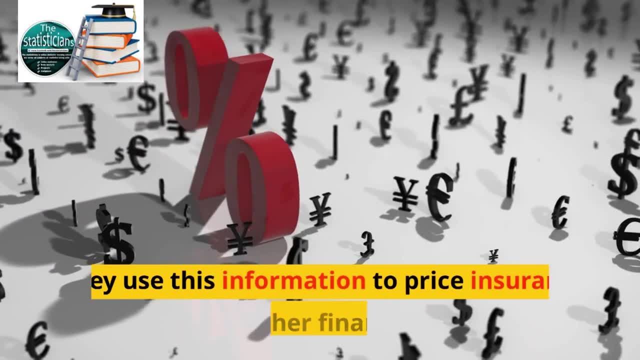 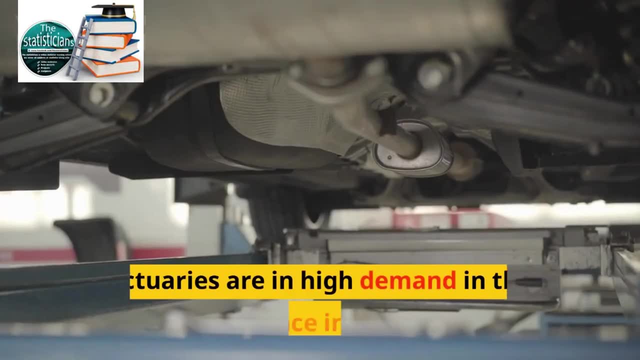 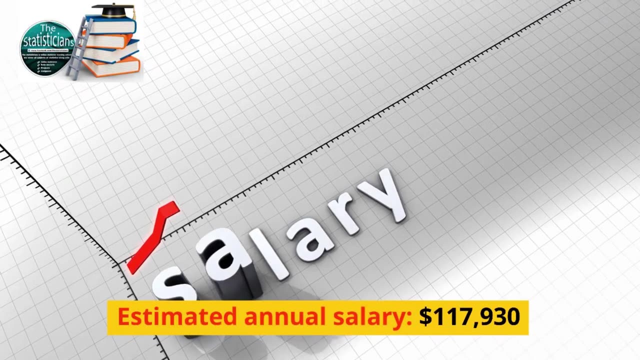 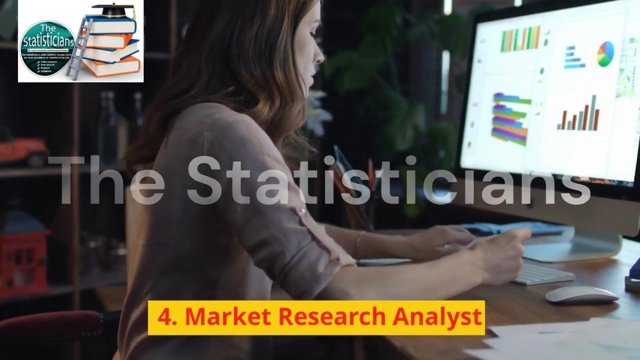 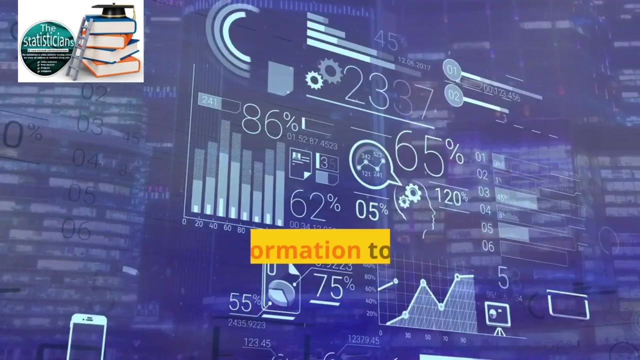 uncertainty. They use this information to price insurance policies and other financial products. Actuaries are in high demand in the insurance industry. Estimated Annual Salary – $117,930. 4. Market Research Analyst. Market research analysts collect and analyze data about consumers and markets. They use 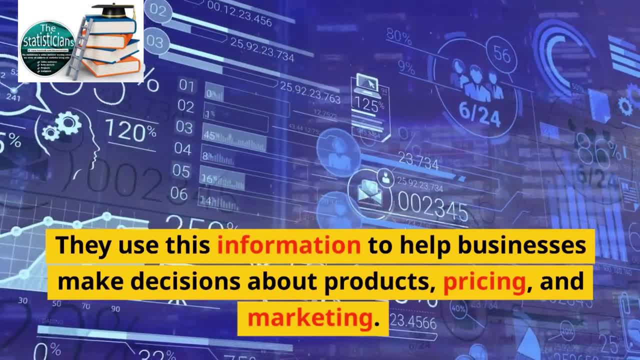 this information to price insurance policies and other financial products. Actuaries are in high demand in a variety of industries, including business, healthcare and government. They use this information to falsify analysis deemed to be unethical or rob a lot of financial. 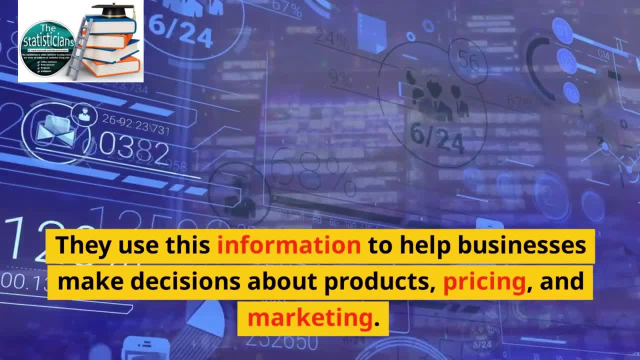 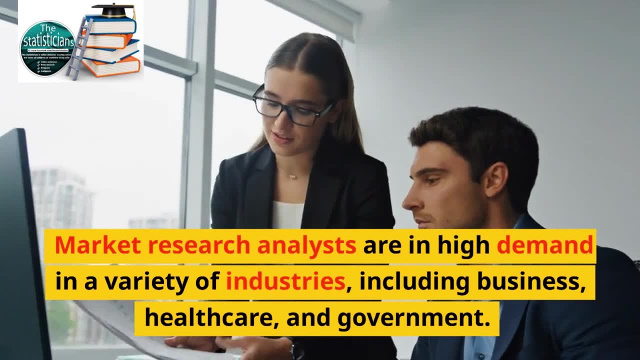 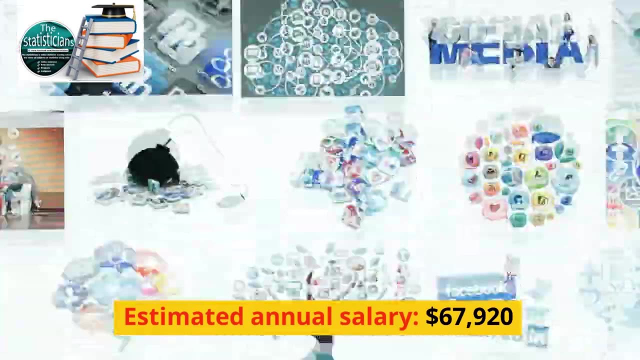 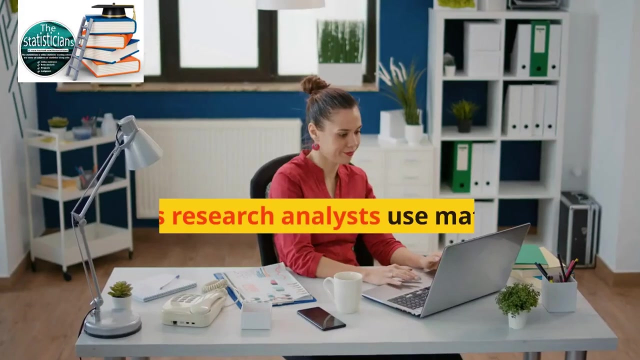 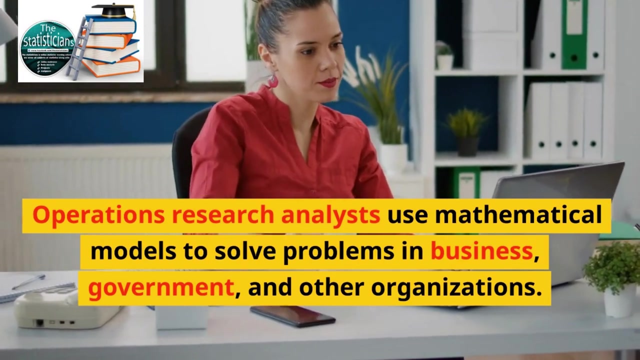 debt or치 citizen בעatan. Estimated Annual Salary: $67,920. 5. Operations Research Analyst. Operational Research Analysts use mathematical models and data to test their Impact. presenters to solve problems in business, government and other organizations. They use this information to improve efficiency, productivity and profitability. 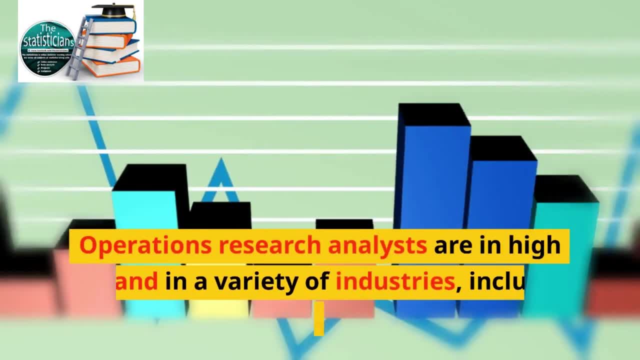 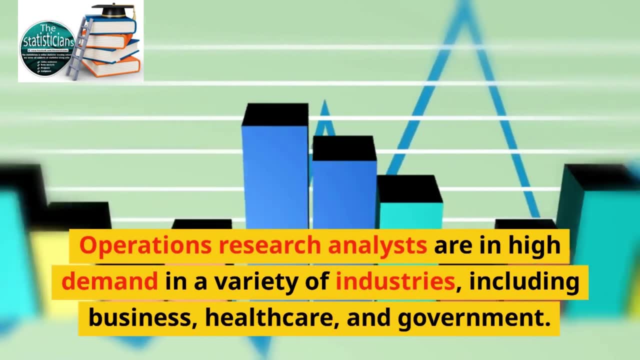 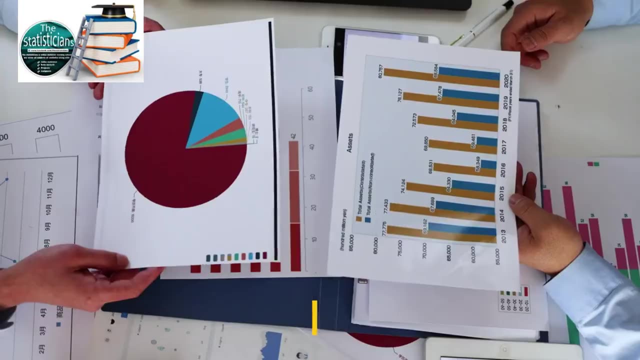 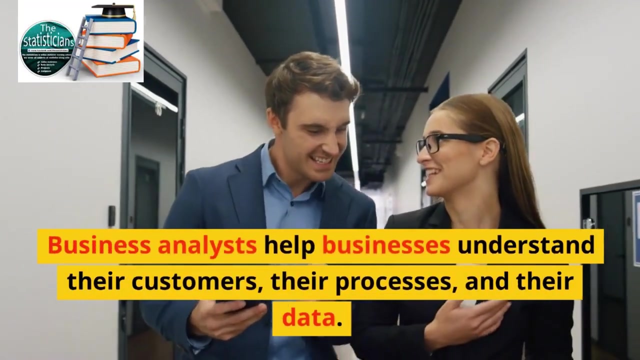 Operations. Research Analysts are in high demand in a variety of industries, including business, healthcare and government. Estimated Annual Salary: $89,190. Sex Business Analysts. Business analysts help businesses understand their customers, their processes and their data. They use this information to make recommendations for improvement. 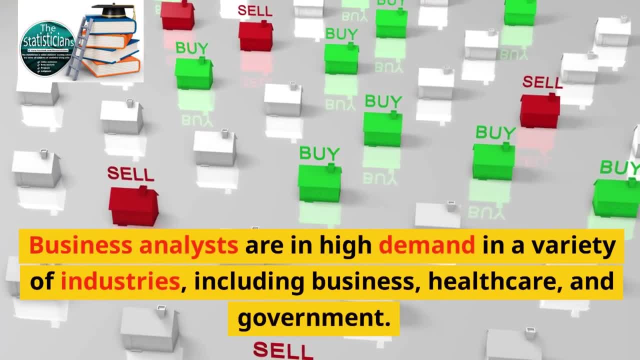 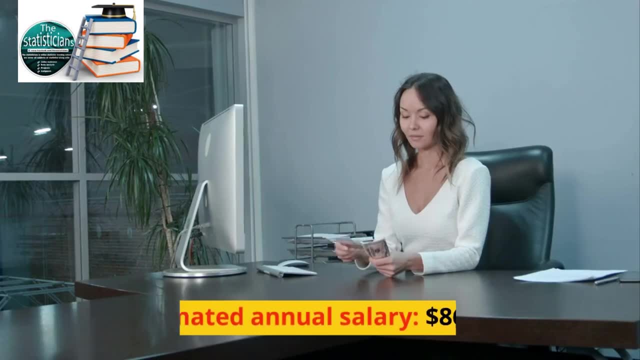 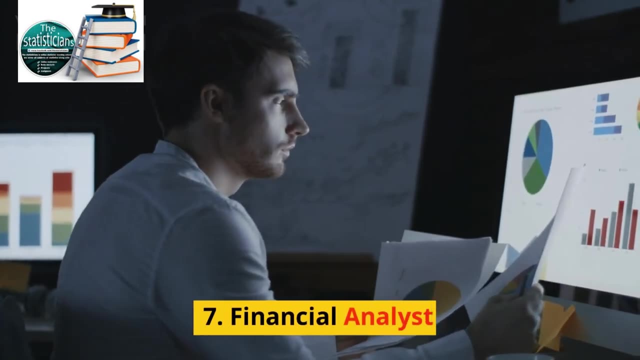 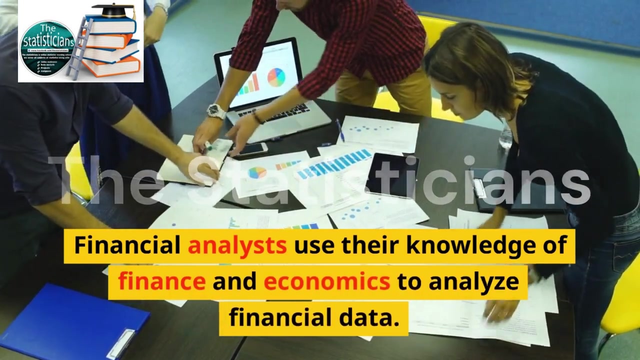 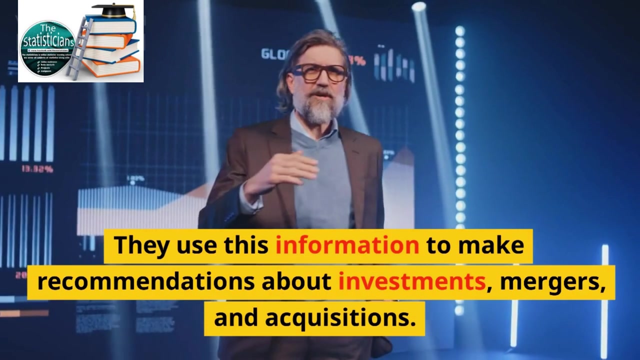 Business analysts are in high demand in a variety of industries, including business, healthcare and government. Estimated Annual Salary: $86,270. Financial Analysts: Financial analysts use their knowledge of finance and economics to analyze financial data. They use this information to make recommendations about investments, mergers and acquisitions. Financial analysts are in high demand in the financial industry. Estimated Annual Salary: $82,190. Risk Analysts: Risk analysts assess the risks associated with a variety of activities, such as investments, projects and operations. They use this information to make recommendations about how to mitigate risk. 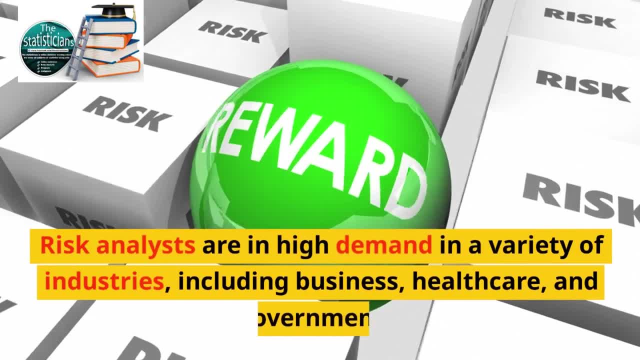 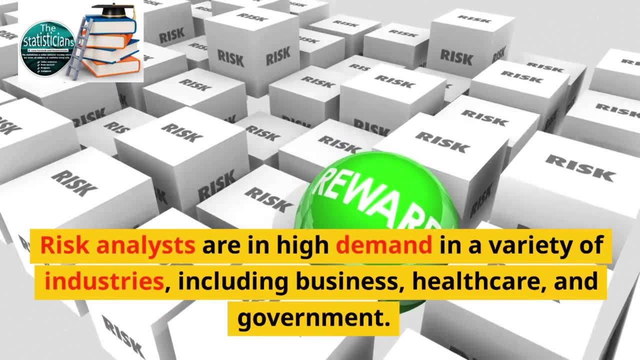 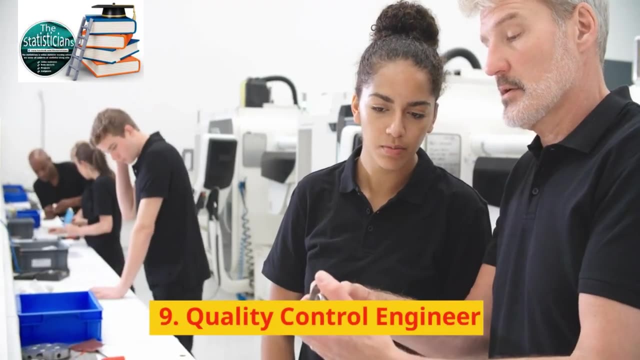 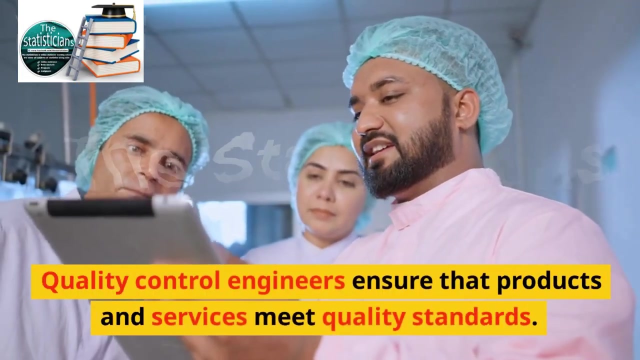 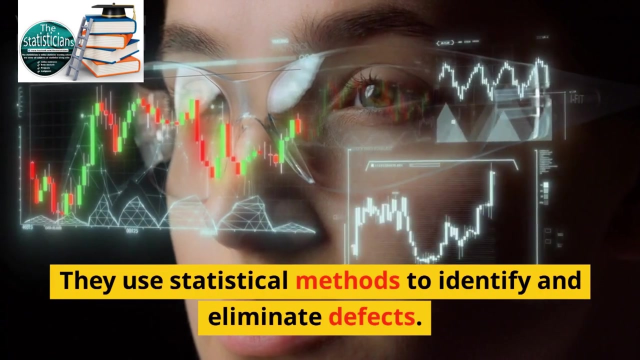 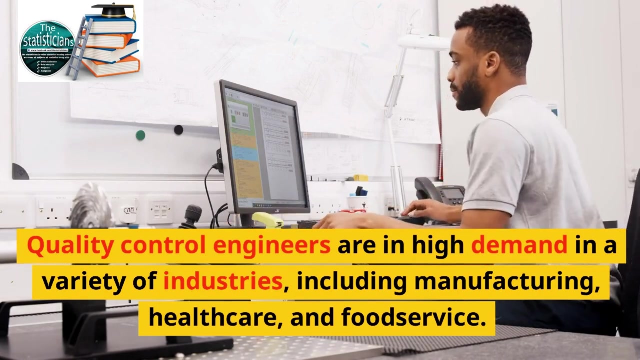 Risk Analysts are in high demand in a variety of industries, including business, healthcare and government. They use this information to make recommendations about how to mitigate risk and how to mitigate risk. Risk Analysts' Turbulence Risk Analysts- variety of industries including manufacturing, healthcare and food service. Estimated annual. 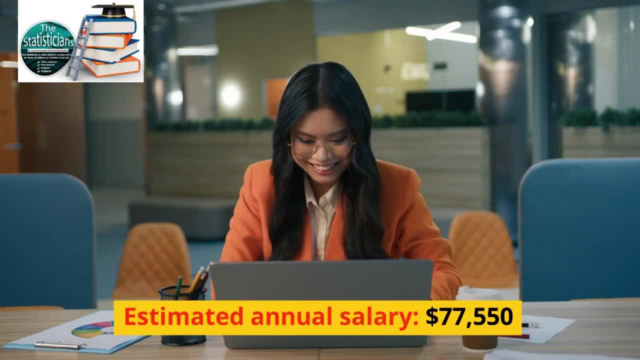 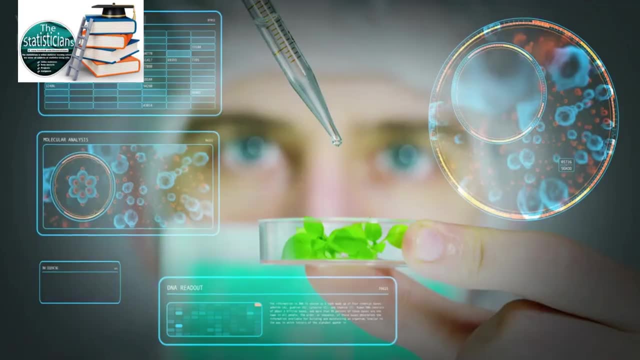 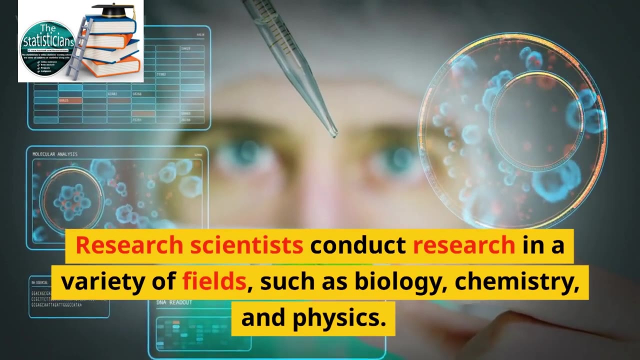 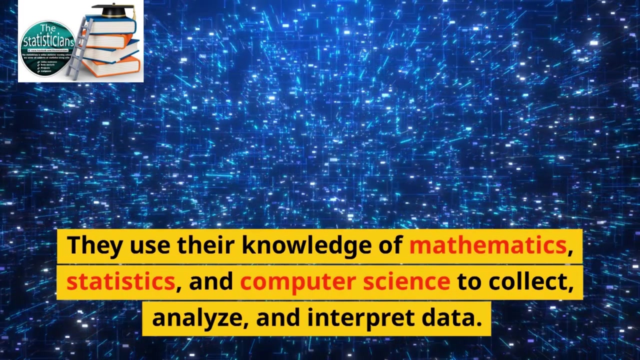 salary: $77,550.. 10. Research Scientist. Research scientists conduct research in a variety of fields such as biology, chemistry and physics. They use their knowledge of mathematics, statistics and computer science to collect, analyze and interpret data. Research scientists are in high